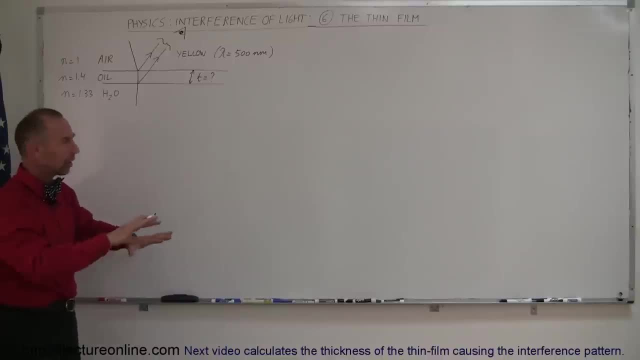 of the puddle, you see all kinds of different colors, different rings of colors shining everywhere, And so let's say that in our example, there's an observer looking down at a particular spot on the oil and sees yellow light being reflected off the film, and the question is how? 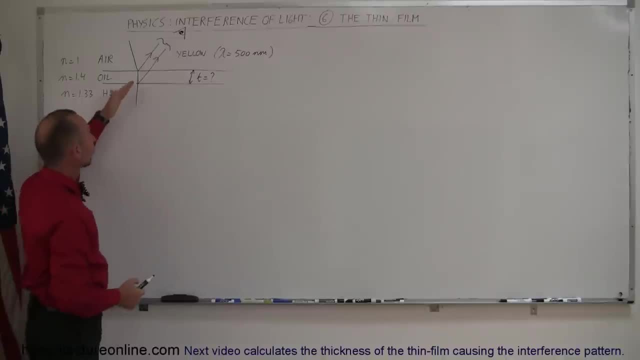 thick should the oil film be in order for the observer to see yellow light being reflected back? if sunlight is entering upon this, this puddle, And of course the sunlight will then have all the various colors of the rainbow distributed throughout it and only the yellow light is. 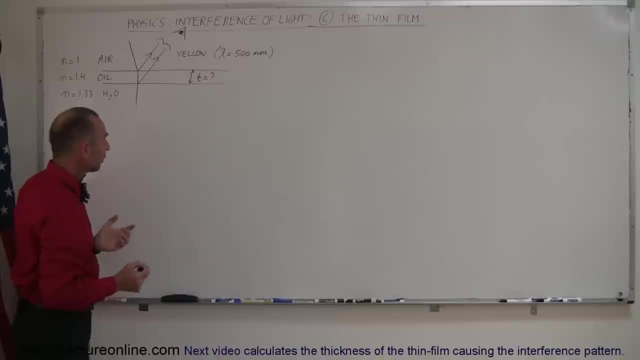 being reflected. So what is the thickness of the oil? So, again, the first thing you do is: okay, that means that theéd second ray that goes all the way through the oil and is reflected off the boundary between oil and water, That has to travel an extra distance and it looks like the extra distance. 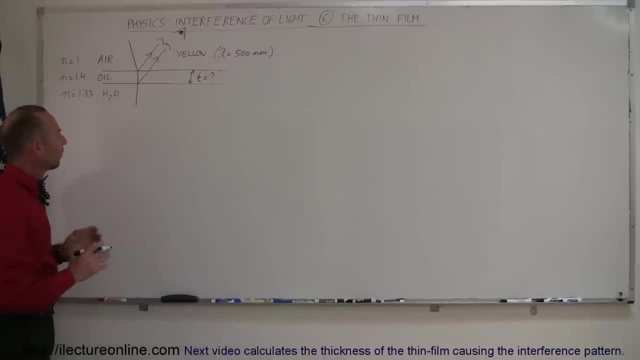 is equal to twice the thickness of the oil. You say, well, wait a minute, that angle doesn't look like it's more than twice the thickness. and yes, it is, but I just drew it like that so it's easier to see. Let's just assume that these angles are so small that we don't have 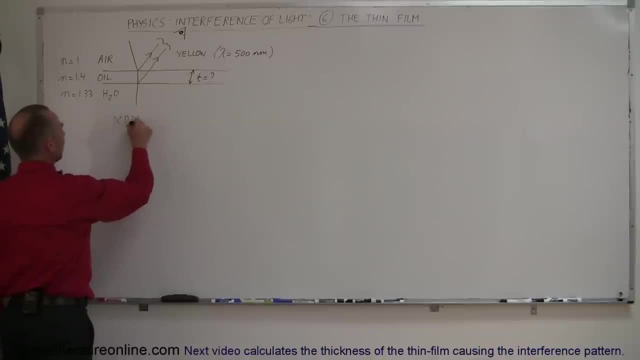 to worry about them. So we can say that the extra distance traveled is equal to twice the thickness of the oil. and, of course, for yellow light to be reflected, you want the phase difference for that yellow light to be zero. In other words, you want the extra. 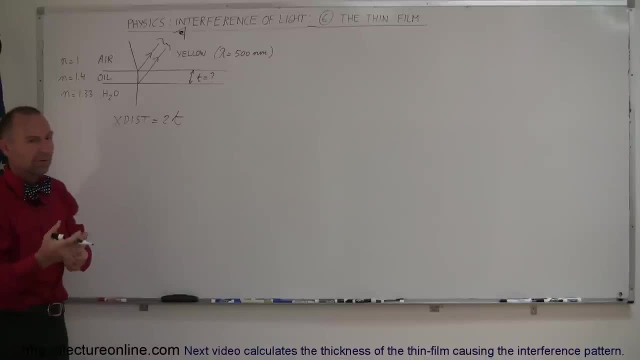 distance traveled equal to be a full wavelength or two wavelengths, or three wavelengths or so forth. However, before we go there, let's take a look at these boundaries and determine if there was a phase shift, And notice a phase shift when light is reflected off a boundary. 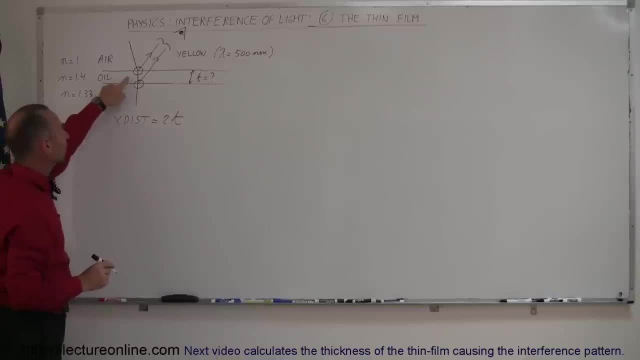 will always occur when the index of refraction on the other side is greater than where the light came from. In this case, it came from air And when the boundary was on the other side is oil, so the index of refraction is greater. 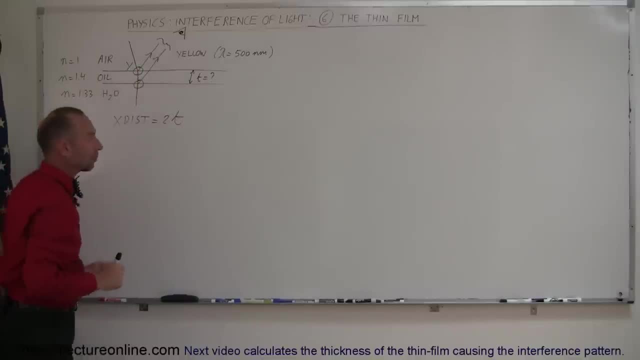 and we can say, yes, there was a phase shift at this particular boundary. Then we get to the other side, where we have the boundary between oil and water, and here the index of refraction on the other side is smaller than it is where the light came from. So here there, 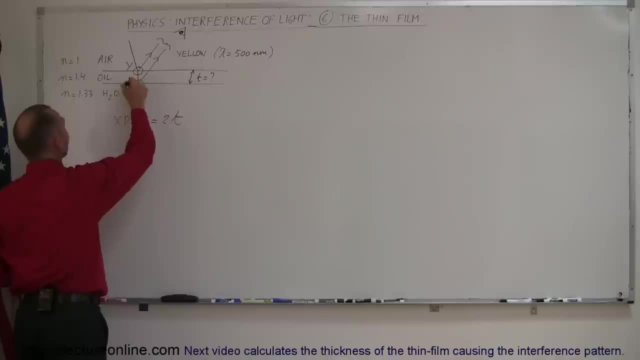 will not be a phase shift, and so we say we write the letter N for no. So yes, there was a phase shift there. no, there was no phase shift there. Which means that the first beam that gets reflected already has an immediate 180 degree flip or a half wavelength flip. The second 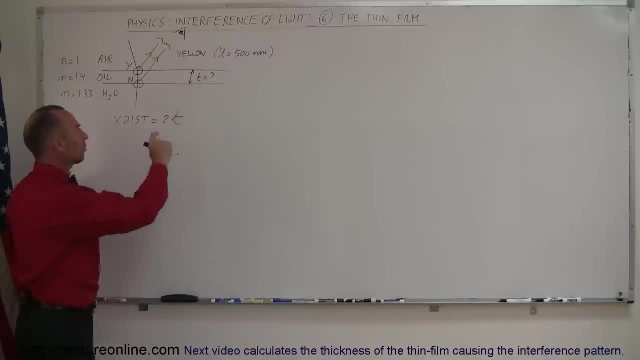 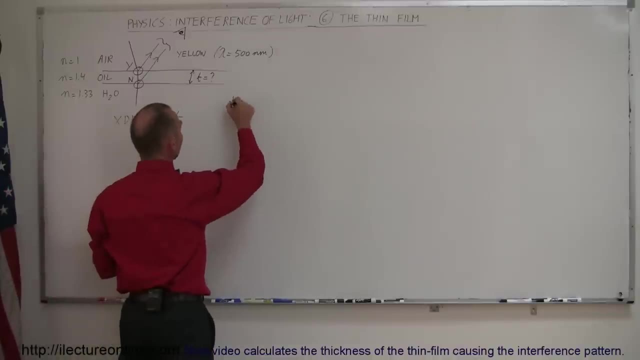 beam does not not have a wavelength shift. That means if the extra distance traveled was zero, the two ways to would already be 180 degrees out of phase. So let's write that down, for t equals zero. 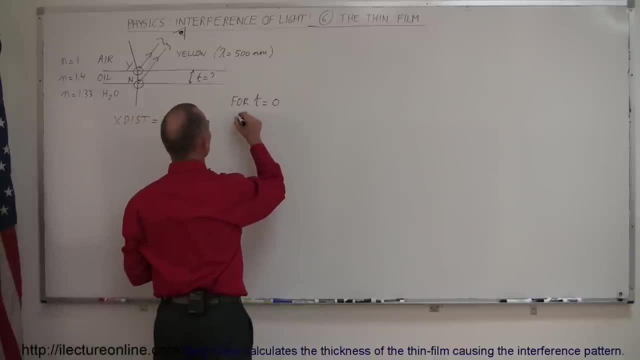 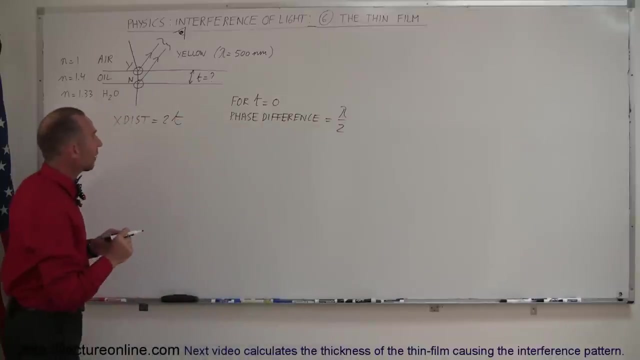 for zero thickness. then the shift in the wavelength or the phase difference. I should say, maybe that's say it- the phase difference is already a half a wavelength. and the reason again, why is it different by half a wavelength? because there is there is a phase shift on the first boundary and no phase. 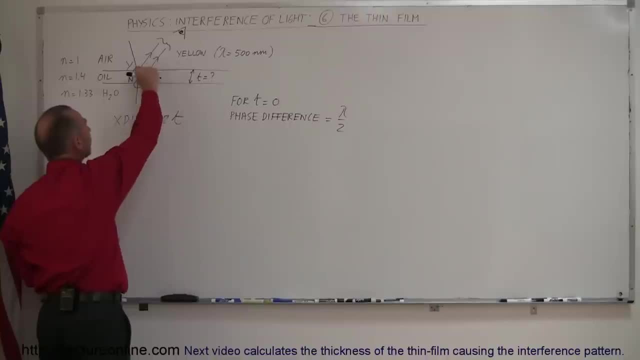 shift on the next boundary. so even if t was infinitely small, they will already be 180 degrees out of phase or half wavelength out of phase. now to get the condition for the two waves to come together here and have constructive interference for yellow light, you want the phase difference. 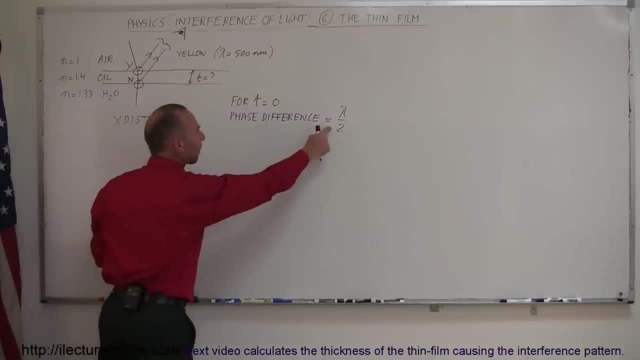 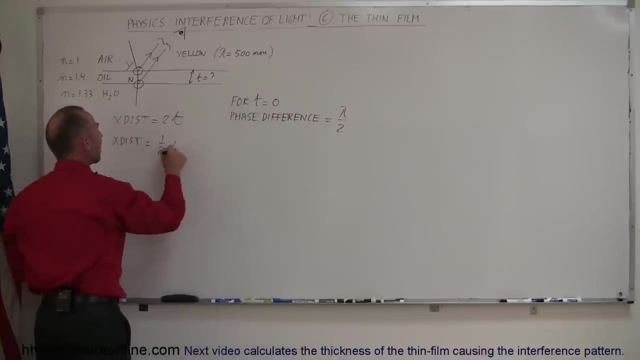 be a full wavelength. that means you only need to make up the other half a wavelength, which means the extra distance traveled must therefore only be a half a wavelength through the oil instead of a full wavelength. so that means that twice the thickness of the film must be equal to a half. 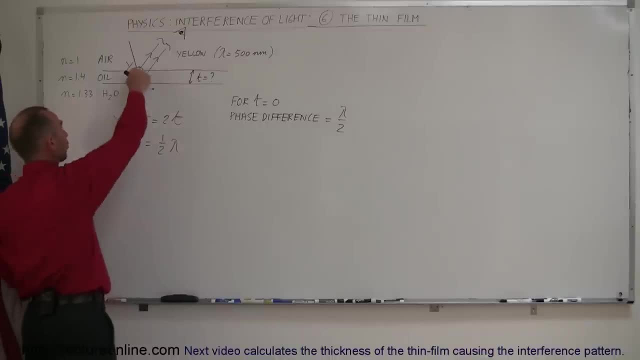 a wavelength. not only that, since the light is traveling through oil and the index of refraction is not equal to one, we have to make sure that we take into account that the wavelength will be different as it travels through the oil. so this will be equal to one over or one lambda. let me just write it like this. so well, it's right. 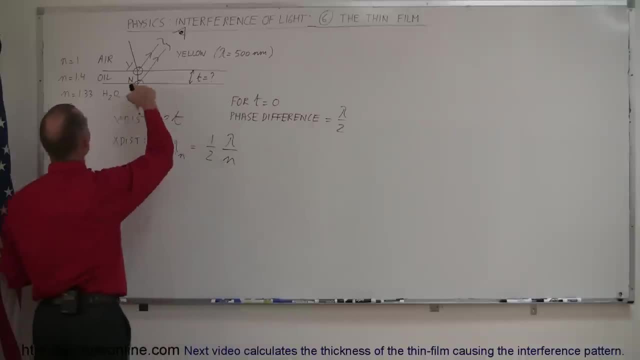 at least one half lambda divided by n, where n is the index of refraction of the oil. now we're ready to go. so now we determined that the extra distance travel should only be a half a wavelength, and is the wavelength of the lightness that travels through the oil, and then we set those two equal.